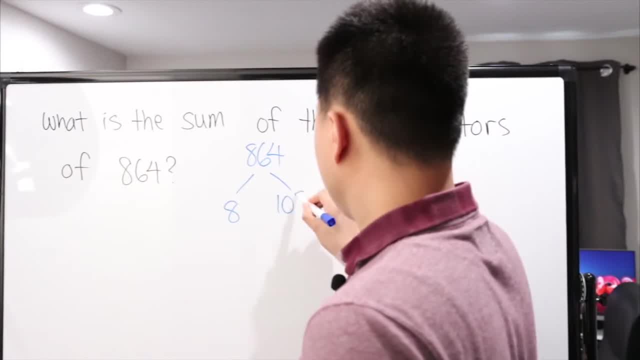 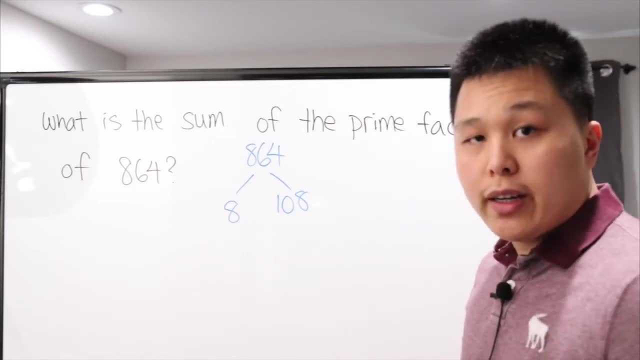 this down into 8 and 108. And here you guys can either check with the divisibility rule, or if you guys end up breaking it down in a different way, that's entirely fine. As long as we break it down correctly, the end result should still be the same. Well, we? 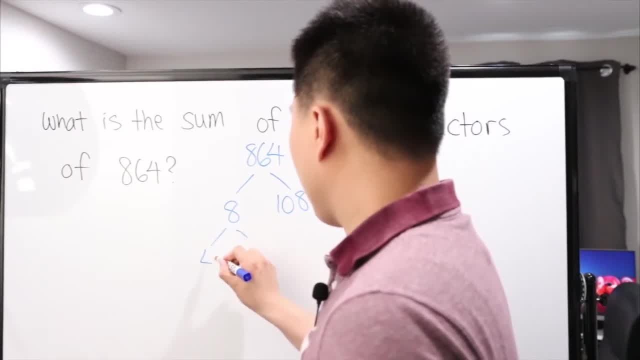 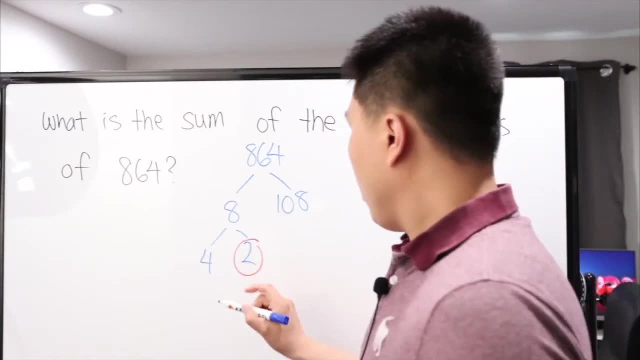 know from our experience, 2 is a prime. so here we go. We're going to just mark it so that we know we're done. 4 can be broken down into 2 and 2.. There we go, And so we're going. 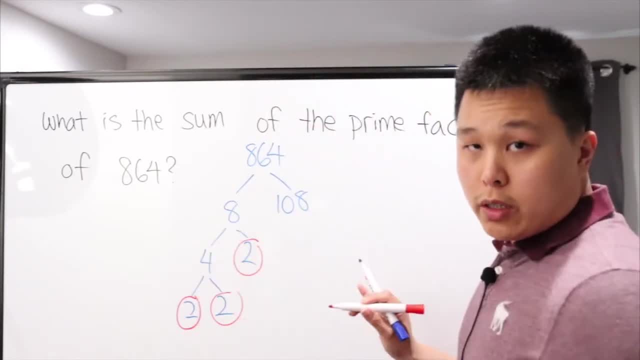 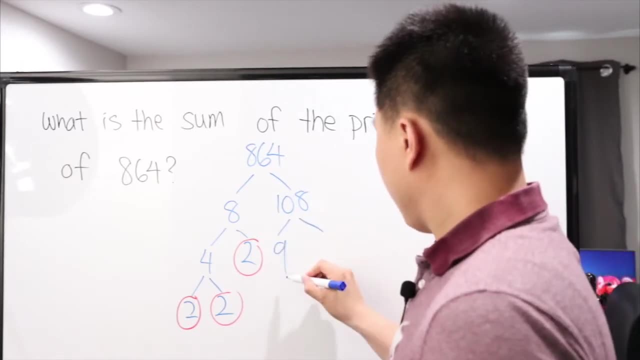 to mark those guys down. So this whole side- right here we're done- Finished. Now we got to worry about this one Here. 108 from our experience can be broken down into 9 and 12, I believe. So we have 9 and 12.. 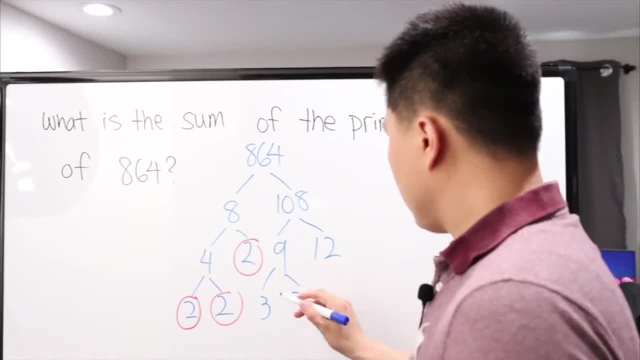 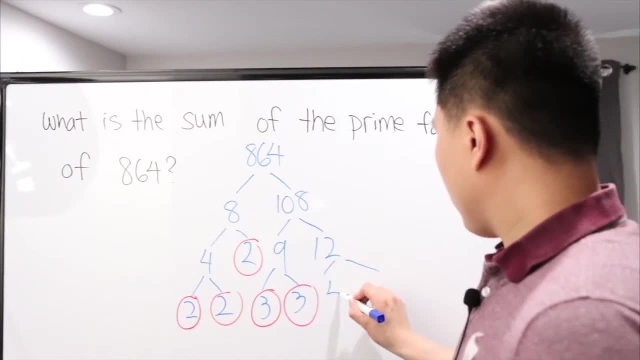 Well, in this case, 9 can be broken down into 3 and 3. So we have 3s as primes- and that's just from our experience- And 12 can be broken down into 4 and 3.. Here this 3. 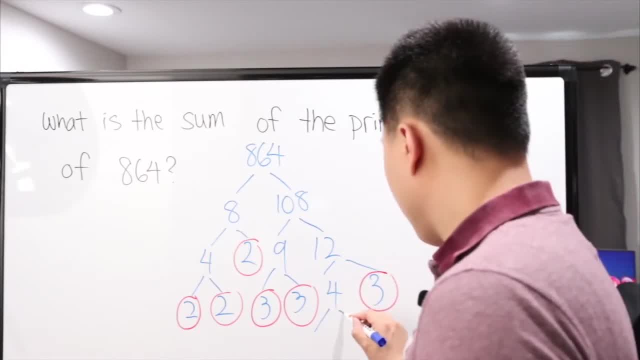 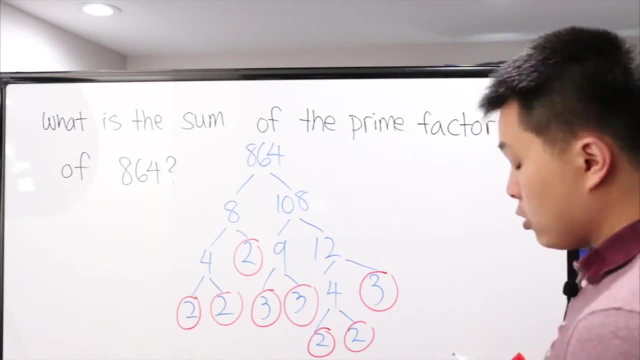 is a prime as well. And lastly, we have 4, which we can break it down into 2 and 2.. So those are prime Great. So we followed everything. All of them are prime factors. Good, That. 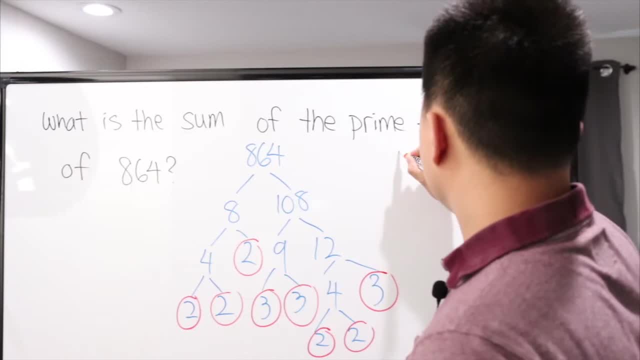 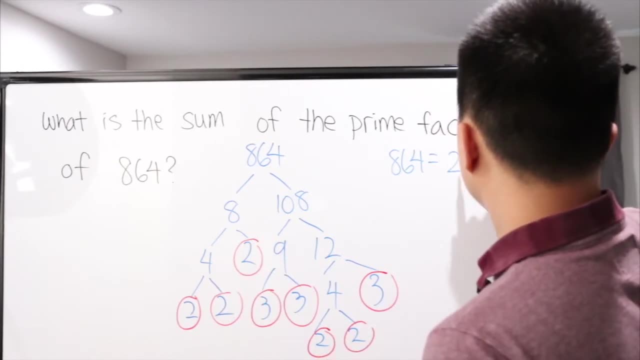 part is done. Now we can rewrite it to make it easier on ourselves. We have 864,, we're done with 864.. And then we have 2 times itself: 1, 2, 3, 4, 5,, 5 times. So 2 to the 5th power. 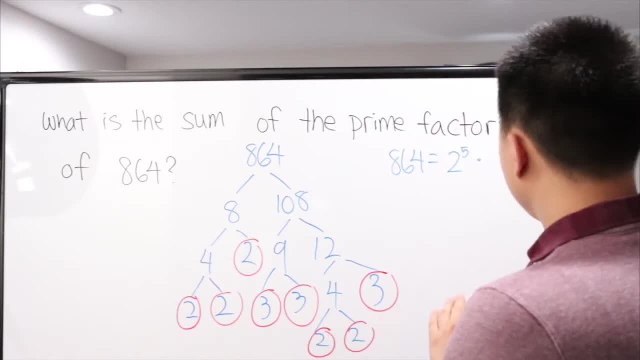 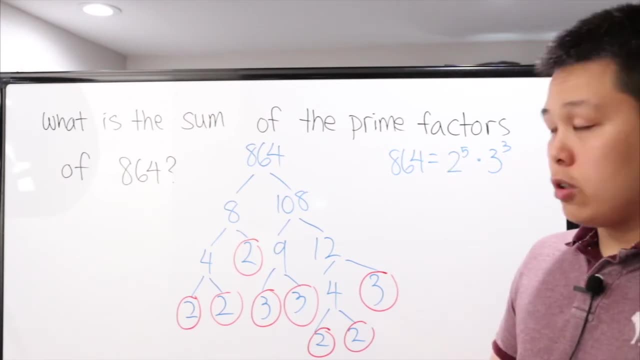 times And we have 3 times itself: 1,, 2,, 3,, 3 times itself, 3 times. There we go. 864 is equal to 2 to the 5th power times, 3 to the 3rd power. Well, in this case the 2 and. 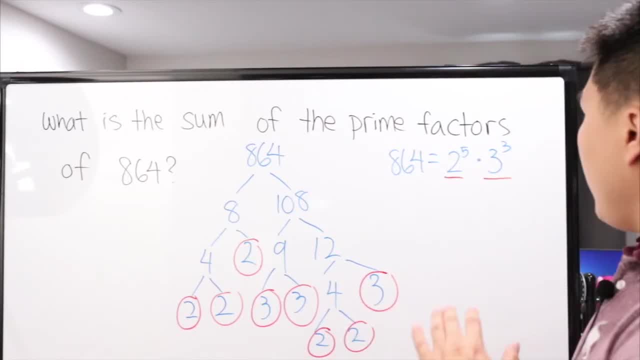 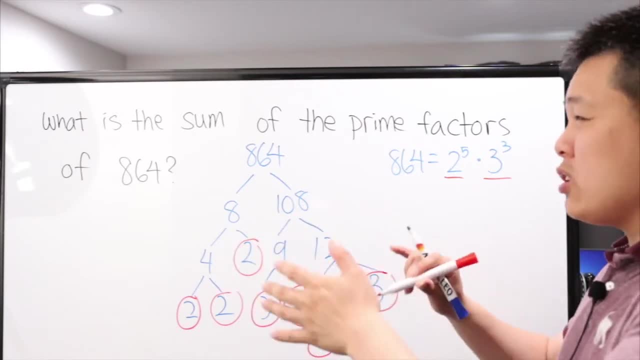 the 3 is our prime factors. Great, Now what do we do next? Well, in this case there's two interpretations. That's where the confusion, that's why I said it's like confusion, complication. however you want to say it comes in. There's two ways. I've seen this. 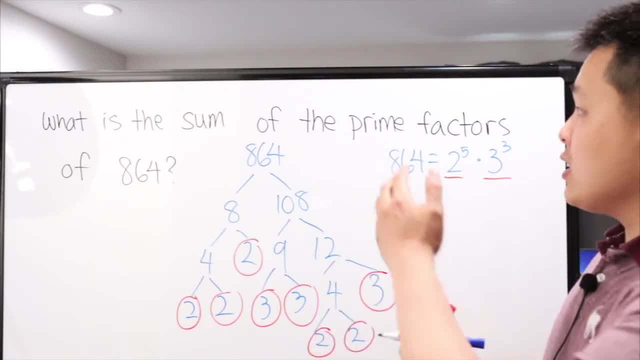 kind of problem interpreted. The first one is that they're assuming the sum of the prime factors is basically the sum of all the unique prime factors. So the unique prime factors in this case is just 2 and 3.. So you would add 2 and 3 together and you would get 5,. 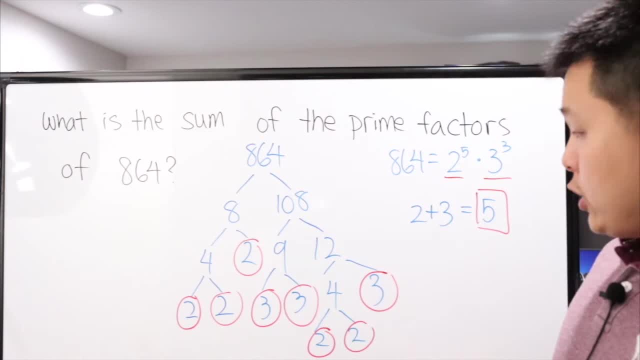 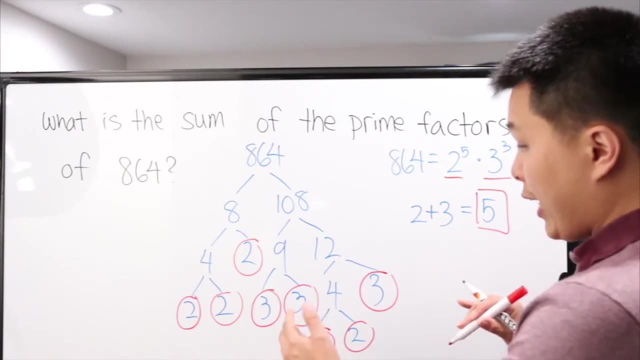 and that would be your answer. Now the other interpretation also makes sense. I find no fault in it. Rather than assuming that they're unique prime factors, we're assuming you know we're going to add each and every one of these individual prime factors. Well, in 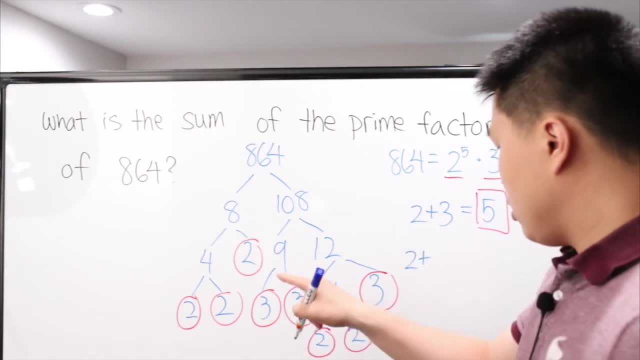 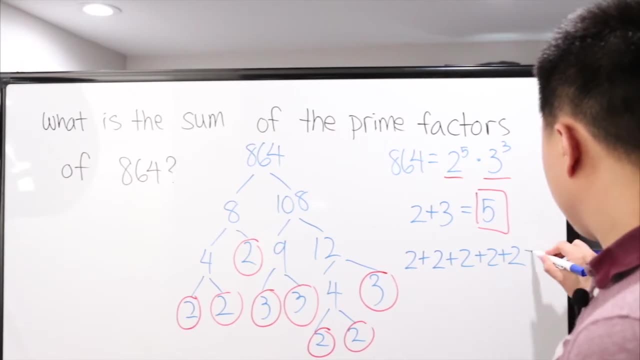 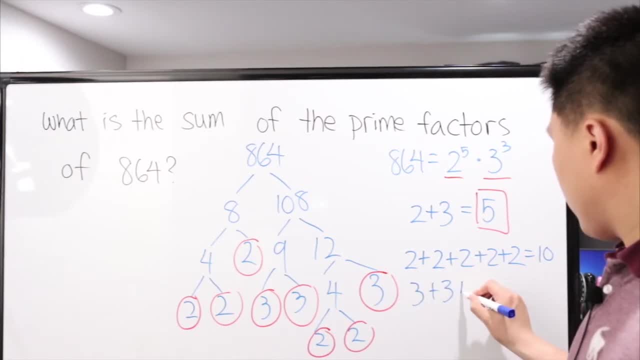 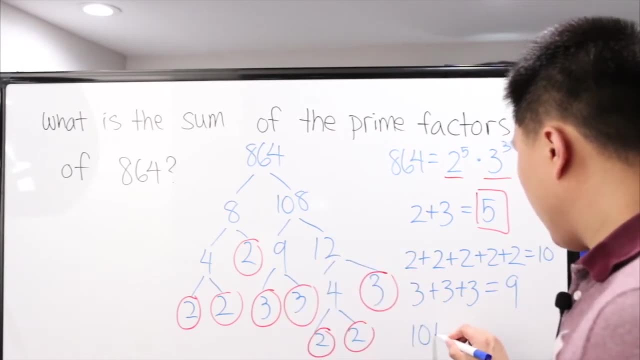 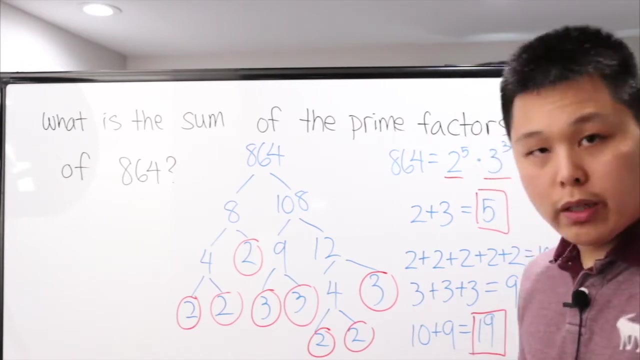 adds itself 3 times 3 plus 3 plus 3, which gives us 9.. And then, of course, we're adding it all together, So we have 10 plus 9. in this case, 6 equals 19. And so that is our second possible answer, right? So now we have two of them. 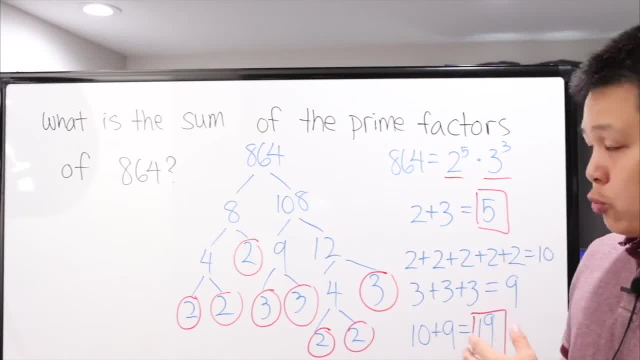 right. This one assuming unique prime factors. This one is assuming all prime factors. We're adding them together. Now, when you encounter a problem like this, especially in a standardized test, you're sort of in luck because usually standardized tests they will give you a multiple. 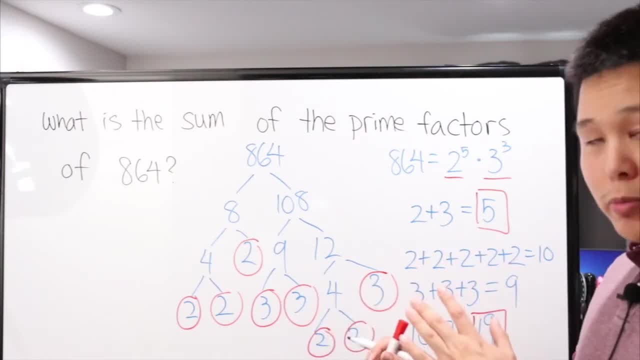 choice Now in the multiple choice, unless the person who designed this problem is just a complete jerk. right The multiple choice, the option is probably going to have one or the other. Now, if you're working on this problem, it's a free response. You can ask the person who. 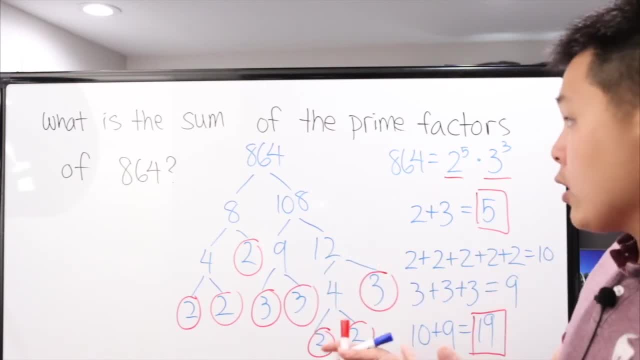 either designed this problem or who is administering this problem- the proctor, for example- what their purpose for this problem is. Do they want the unique prime factors or do they want just addition of all prime factors? And hopefully they'll tell you. If not, then well you. 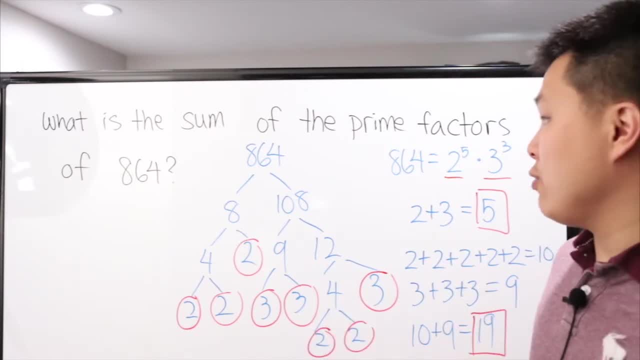 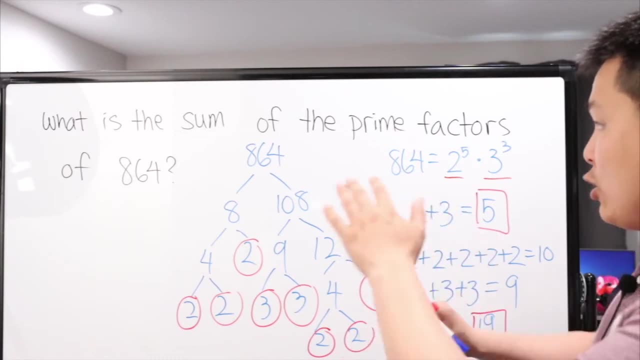 put both of them and then you say it could be either or, and you kind of cross your finger and hope for the best. Well, hopefully this helps And if whoever designs this problem or want to use this kind of problem as a practice, hopefully they are more precise in their language. 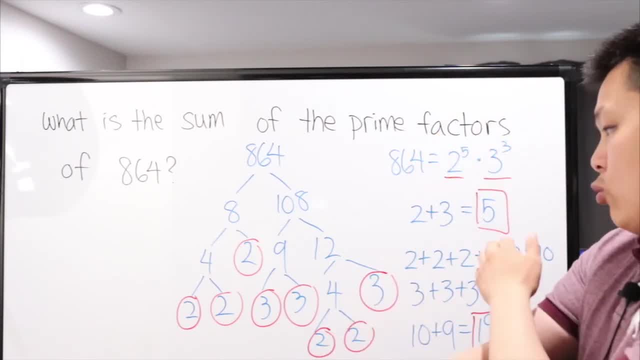 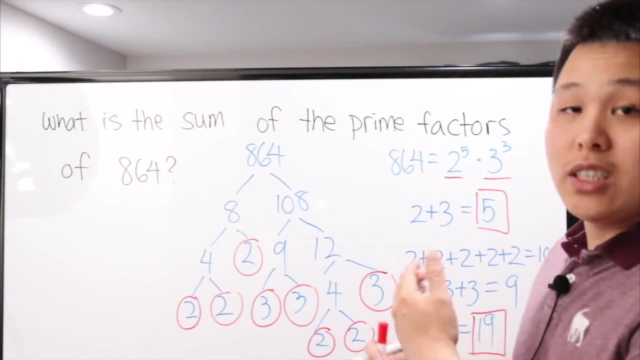 They can specify if they want unique prime factors or if they just want the sum of all prime factors, And then if they change the problem like that, then it would definitely be a lot more easy to understand.